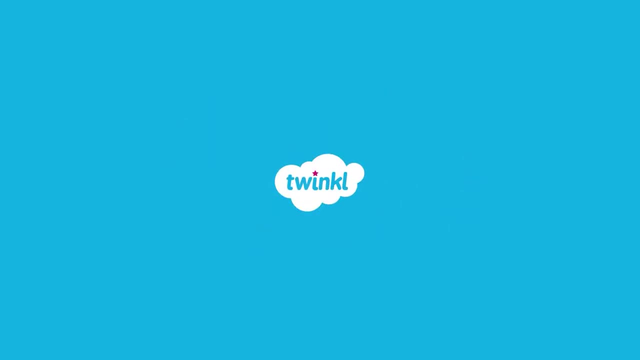 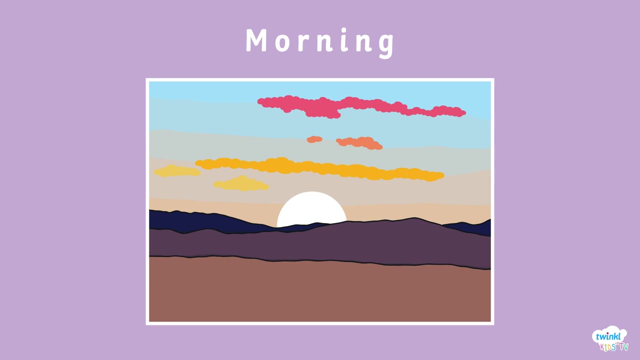 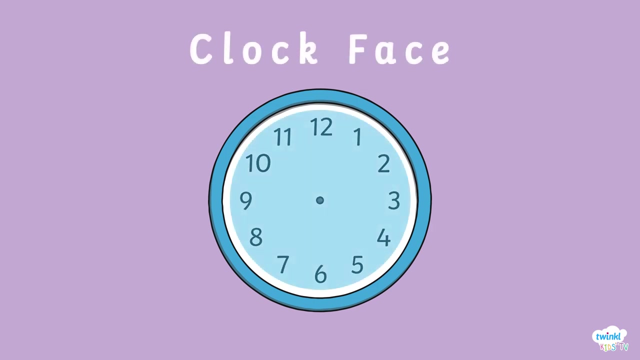 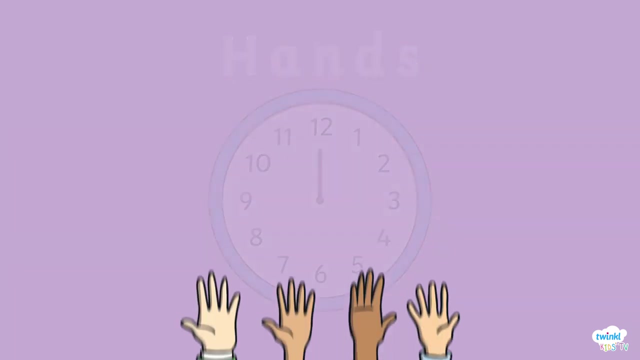 We tell the time so we know when different events happen throughout the day, Whether during the morning, noon, evening or night. This is an analogue clock. The blue highlighted area is called the clock face. The red lines are called hands. No, not these types of hands. We have two. 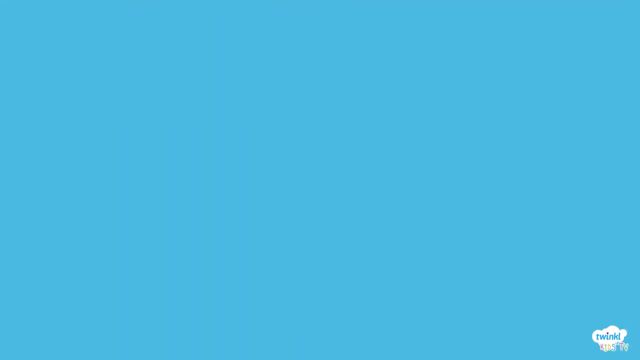 types of hands on the clock. This is the minute hand. The minute hand is the longer hand. The other type of hand is called the hour hand. This hand lets us know what hour it is and it is the shorter hand. The numbers on our clock face represent the hours. Look at the minute hand. 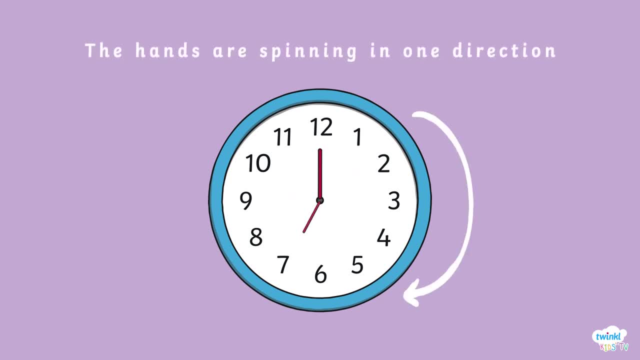 zoom around the clock. We've sped up how long it would usually take- You will notice that both hands are spinning in the same direction. We call this clockwise. What's the time When the longer hand, the minute hand, is pointing to the number 12 and the smaller hand, the hour hand, is pointing to? 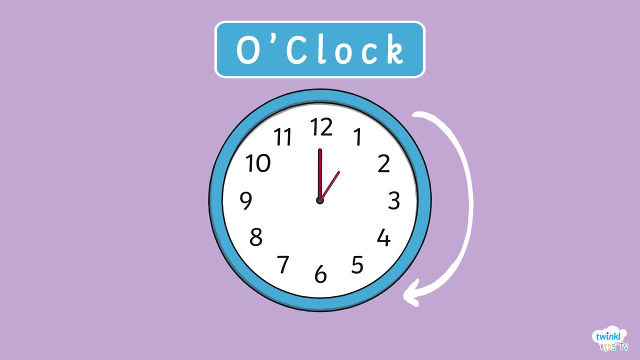 one of the hour numbers. we call this o'clock. For example, when the minute hand points to 12 and the hour hand points to 1, we say it's 1 o'clock. But when the minute hand, the bigger hand, gets to the 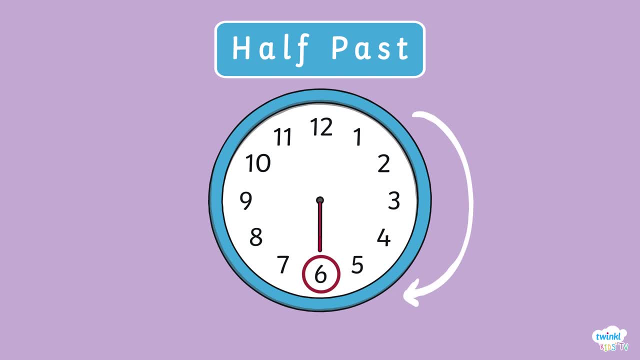 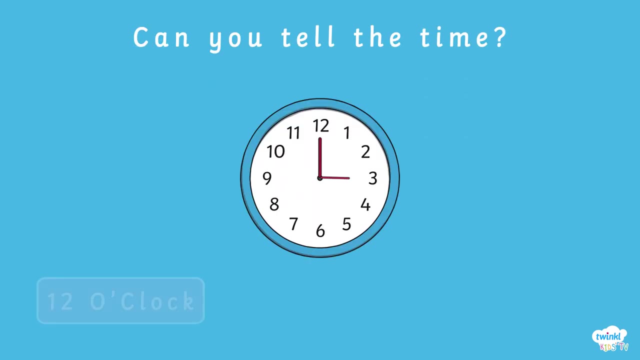 6, then we say half past. You can see that when the minute hand is pointing to the 6, our hand is pointing to the number 7, we say the time is half past 7.. Can you tell the time? Is it 12 o'clock? 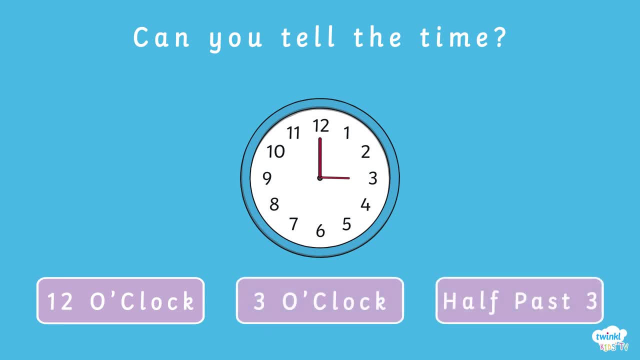 3 o'clock or is it half past 3?? It's not half past 3.. It's 3 o'clock. What time is it now? Is it 10 o'clock, half past 12, or is it 12 o'clock? 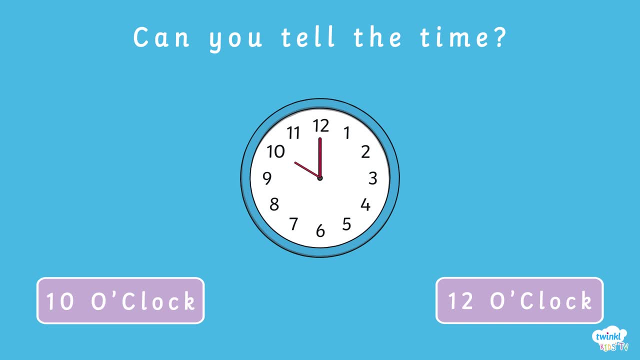 It's not half past 12.. Hint, Look at where the minute hand is pointing: It's 10 o'clock. The big hand is pointing at 12, so we say o'clock and put it after the number that the small hand is pointing to, which is 10.. That means it's 10 o'clock.